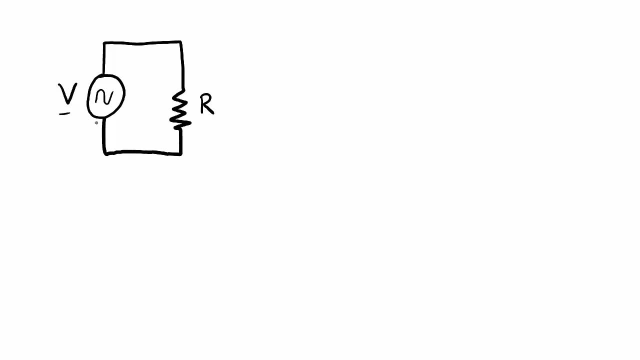 really simple example where I have a voltage source that's an AC voltage source and that's applying a voltage across a resistor. In this simple example, Ohm's law is still going to hold: true Voltage equals IR. or if I'm looking at this circuit where I have a known voltage and a known 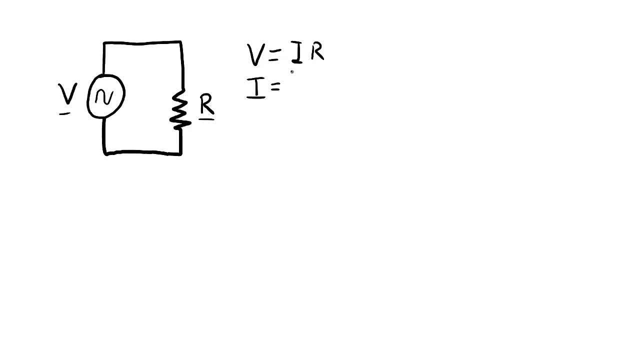 resistance, the current that I will have through that resistor will be equal to the voltage divided by the resistance, or I can write it out as: resistance is equal to the voltage over the current. So, considering that this is an AC voltage, and let's say that it's a voltage that has a 3. 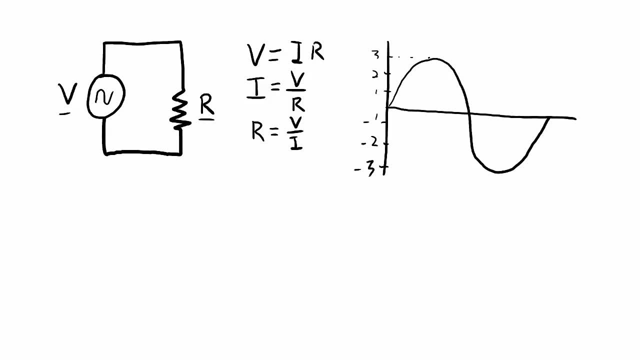 volt peak value, at every instant in time Ohm's law is going to apply. Now, if this is a 2 ohm resistor and I have a 3 volt peak applied, I can say that at every point in time I can apply this. 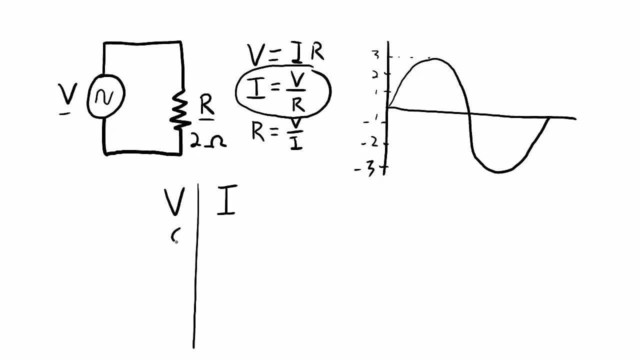 version of Ohm's law to calculate the current. So at the time when the voltage is 0, the current is also going to be 0. When the voltage is 1 volt, then the current is going to be 1 over 2, or it. 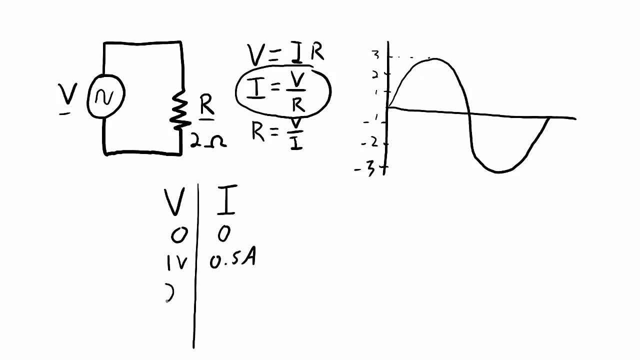 will be 0.5 amps When the voltage is at 2 volt. it will be 0.5 amps When the voltage is at 2 volt, 2 over 2, I will have a current of 1 amp, And when the voltage reaches its peak at 3 volts. 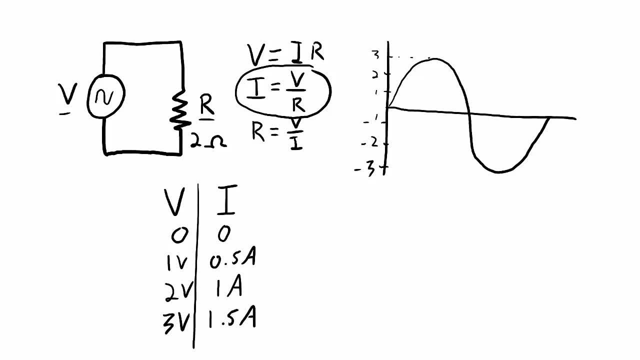 I'll have a current of 1.5 amps And of course this table just represents four points along the whole curve, but it's a continuous curve, so that current is going to be defined everywhere. But let's just look at these four points. So when the voltage is 0, the current is 0.. When 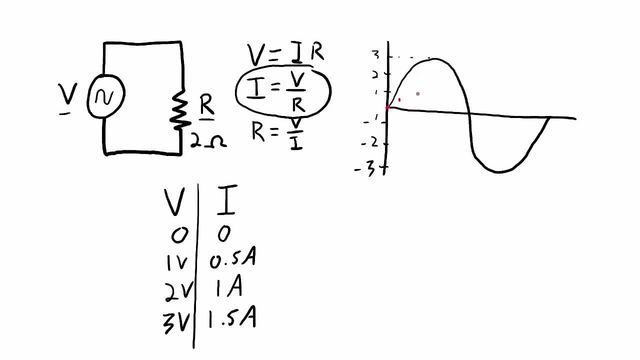 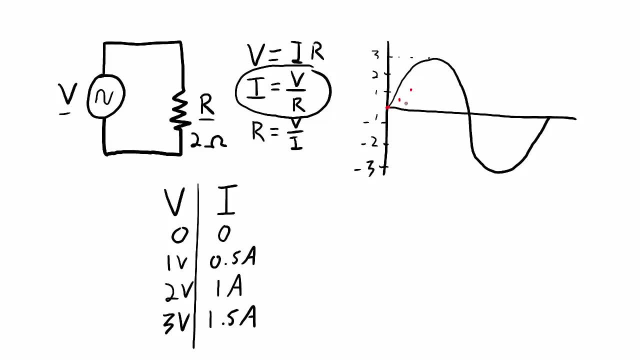 0.5.. When the voltage is 2, the current will be at 1, 0.5.. When the voltage is 2, the current will be at 1,. when the voltage is at 3 volts, the current's going to be at 1.5, and I didn't include negative. 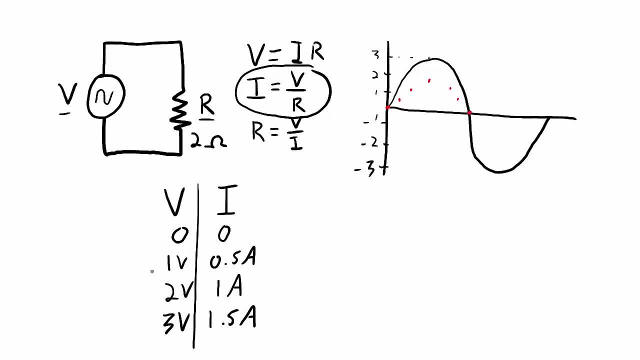 on this in this table. but I could just put a negative sign in front of these and the table would still be true. so when the voltage is at minus 1, the current's going to be at negative 0.5. when the voltage is at minus 2, the current's going to be at negative 1. when the voltage is at 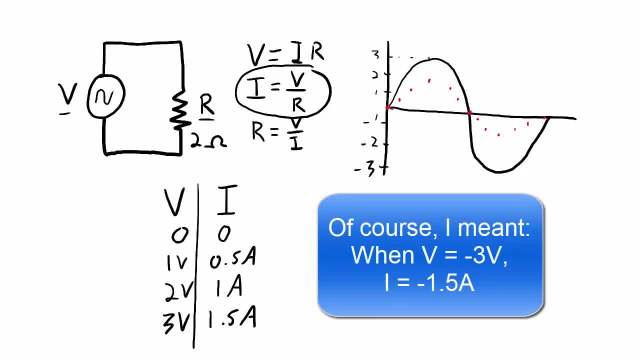 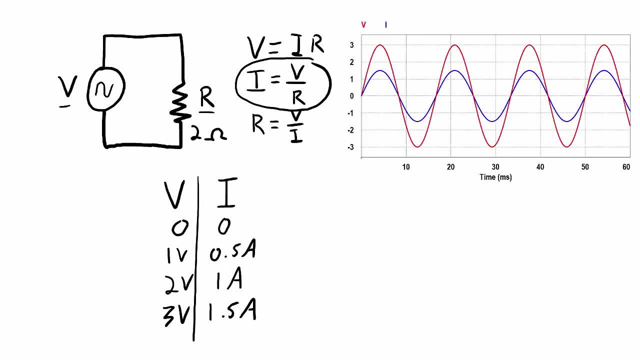 minus 3, the current will be at minus 0.5 and I will get a current curve. if I join all the dots in between- because, remember, it's going to be continuous, I'll get a current that looks something like that, and I've replaced my graph with a much nicer looking one that I've created from a 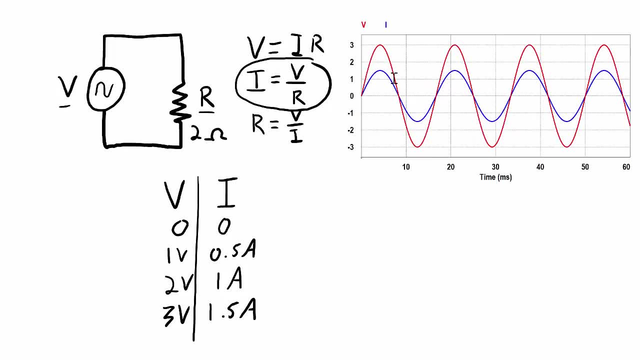 simulation. and voltage is continuous, current is continuous- Ohm's law applies at every instant in time, and so what I end up with is a voltage and a current that are in phase with each other, and since I'm dealing with AC signals, I can write out the voltages and currents for these AC circuits. 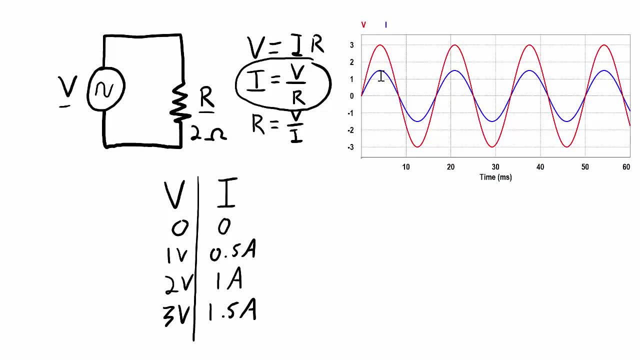 as phasors. So I can use my Ohm's law equations but write them out in phasor form. so the current is equal to the voltage over the resistance. so I can encapsulate all of the information in this table or in this graph here and I can say I can get a 1.5 amp peak current with a phase angle of 0. 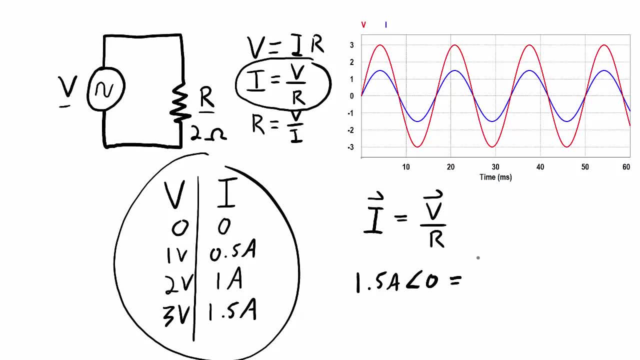 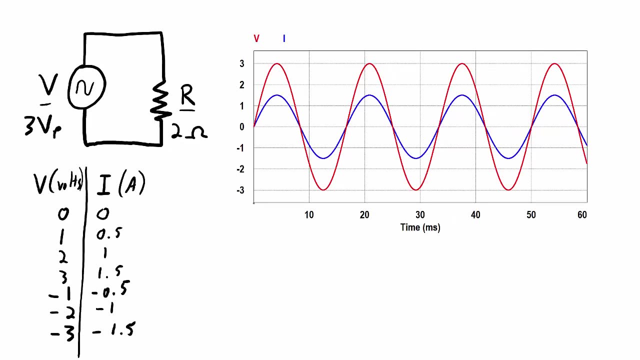 degrees, when I have a voltage of 3 volts with a phase angle of 0 degrees over a resistor which is has an impedance of 2 ohms with a phase angle of 0 degrees. so I've redrawn my circuit here and I've copied the graph of the voltage and current down as well. I've taken the table and 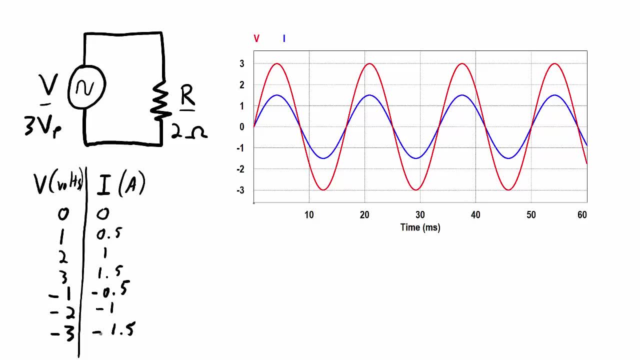 I've added a few points in here. I've added some negative voltages and negative currents because I want to show how power relates. and for any electrical circuit, power is going to be equal to voltage times current. so for each one of these cases, for each one of these values for voltage and 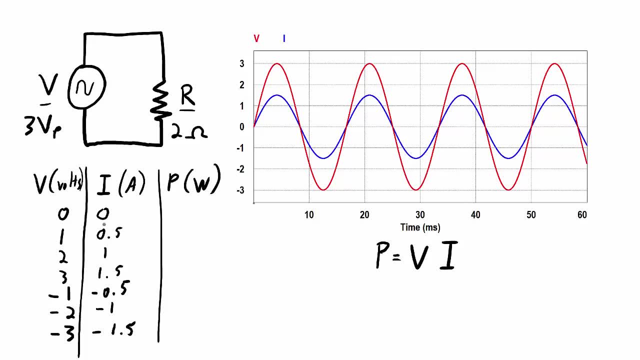 current, I can calculate the power, Which will be in watts. so when both the voltage and current are at 0, the power is going to be 0. here, when I have a voltage of 1 and a current of 0.5, 1 times 0.5 gives me 0.5 watts, 2 volts. 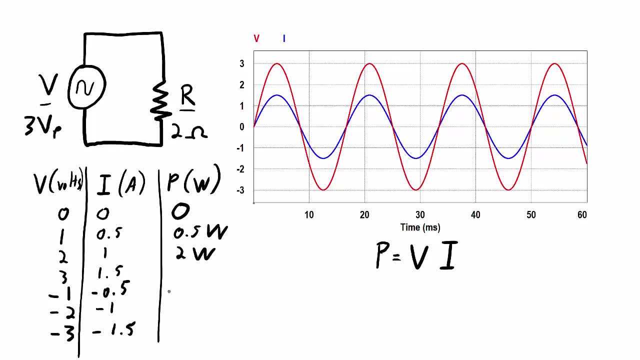 times 1 amp gives me 2 watts. 3 volts times 1.5 amps gives me 4.5 watts. here I get 0.5 watts, 2 watts and 4.5 watts. when the voltage and current are both negative, I get a negative. 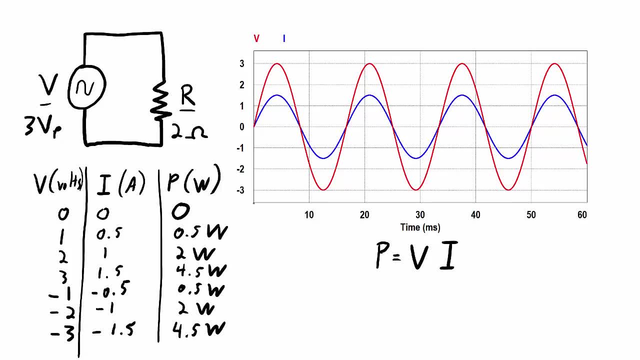 number times a negative number, which gives me equal to 0.5. Positive power. so at every instant in time- maybe a better way of writing this out is: p of t equals v of t times i of t. so so this is saying that as voltage and current vary over time, so does the 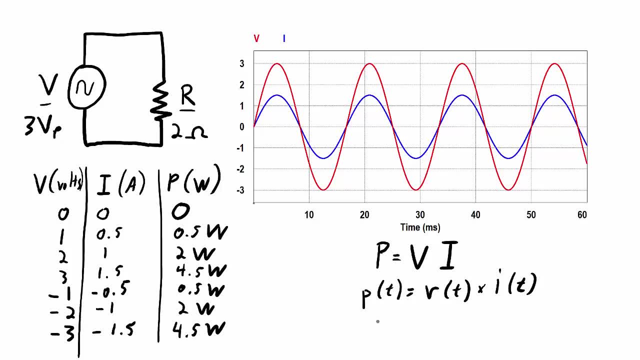 power, and what I can do at every instant in time is take the value of the voltage and the value of the current, multiply them together and I get power. so for these few points I have in the table here, I can plot these out on my graph and then, on the negative side, because I have a negative number times a negative number, it's still. 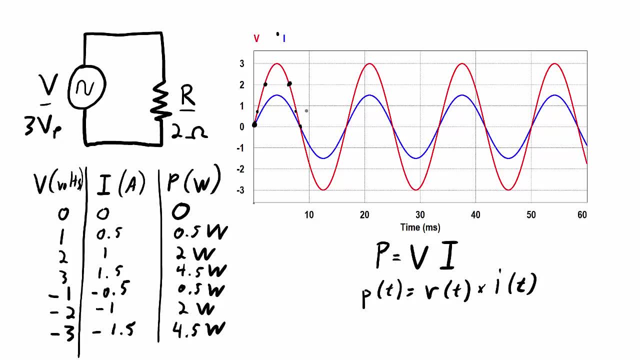 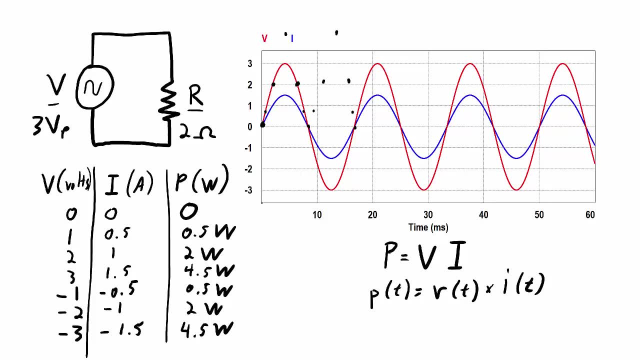 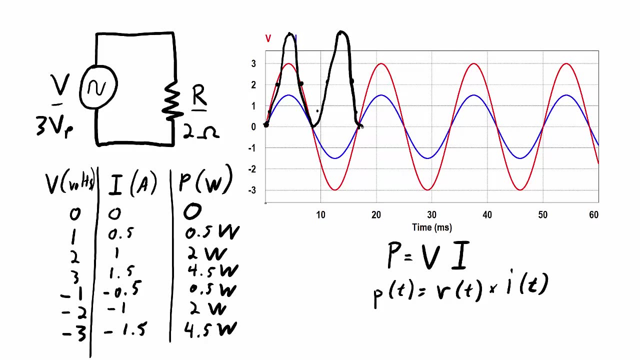 going to be a positive value. so I'll get pretty much the same points and, while it's not so obvious from the few points that I've had, this is going to be a sinusoid, but the difference is that it's not centered on 0 anymore, a sinusoid like that that has a peak and that and it's comes all the. 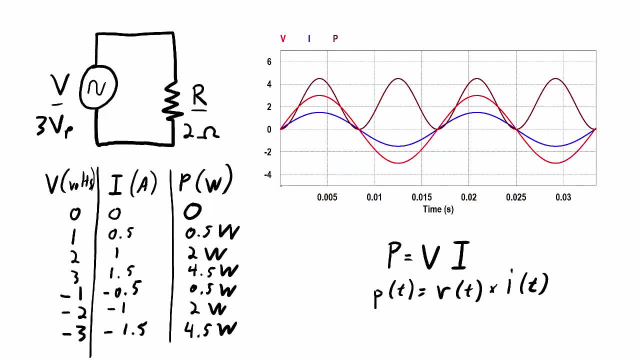 way down to 0 but does not go below 0. here's a much nicer version of this, of that graph that I've created from a simulation. so this is showing the power as it's varying over time. but typically we don't worry about the power at any instant in time. we usually think about 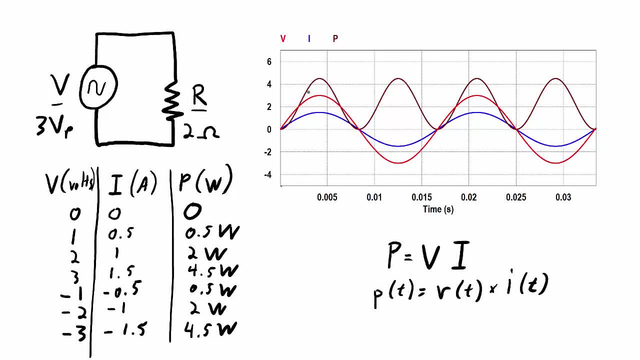 the average power that's being used by a component in the system or the average power that's being delivered by a source in the system and, in general, when you're figuring out the average of something, in this case, the average power, what you're going to do is integrate this signal over one period. 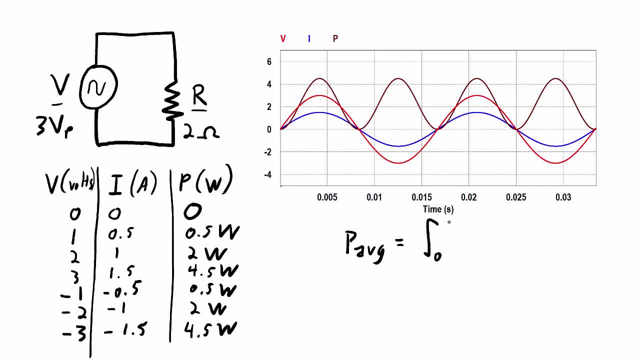 and then divide by the period. so this would be the integral from 0 to t, where t is representing one period. so this would be 1. period here and then divide by the period for a sine wave. this calculation is actually quite easy and if you can read, if you remember or if you think, 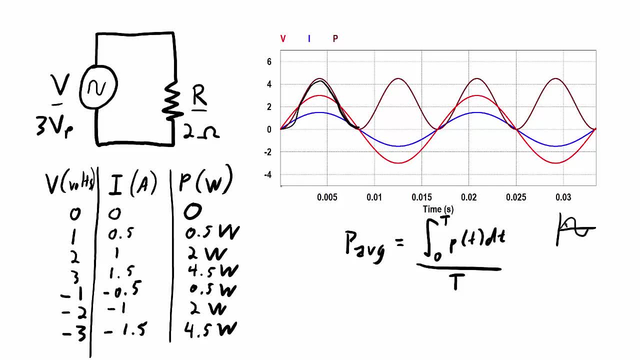 about this. if I have a sine wave that's centered around zero, the area under the curve there and the area and the curve there are equal, but one's positive, one negative, so they cancel out. so the average is halfway between the two positive peak and the negative peak, which in this case is zero. for this case,